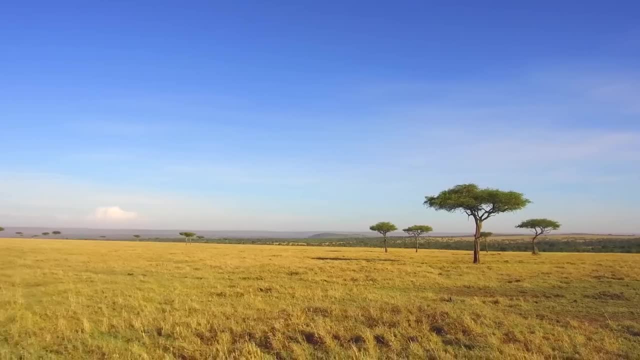 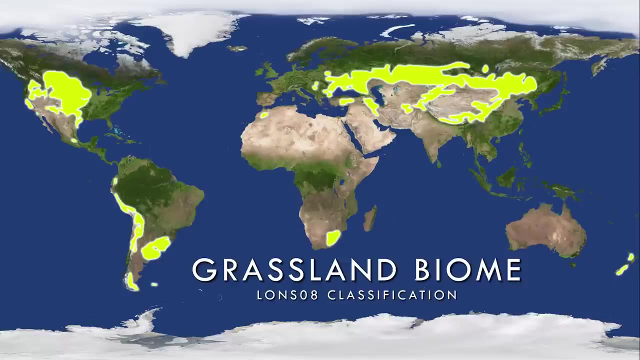 so often confused with grasslands, where we find a mix of grasses, shrubs and trees. Grassland areas occur in relatively temperate, drier climates, either in the mid-latitudes or in high-altitude regions such as the Himalayas and Andes. 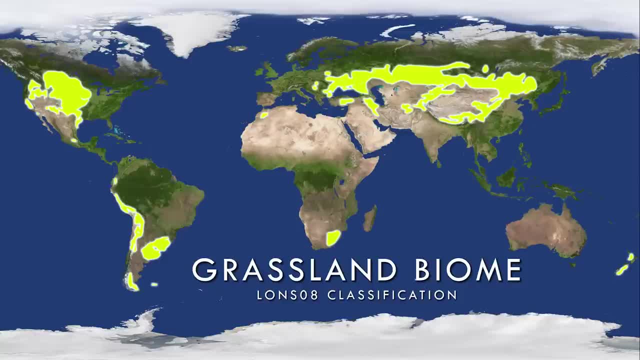 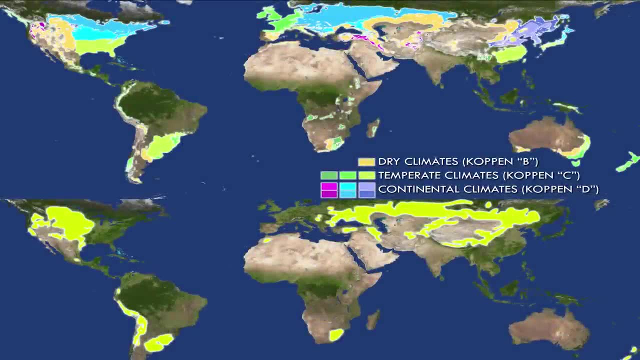 where rainfall is insufficient for tree growth or where historical conditions such as pervasive fire or large animal grazing have prevented trees from gaining a foothold. There is no one Koppen climate type that matches global grassland distribution with continental and cool semi-arid zones. 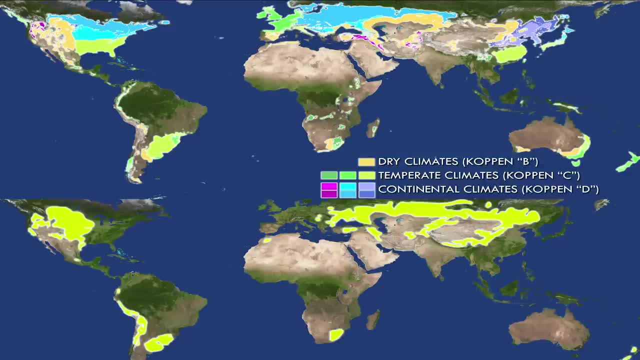 along with humid and highland subtropical zones and even oceanic areas having grasslands. This indicates that the coupling between grassland and climate is not as strong as in the other biomes so far looked at, with major Koppen groups B, C and D. 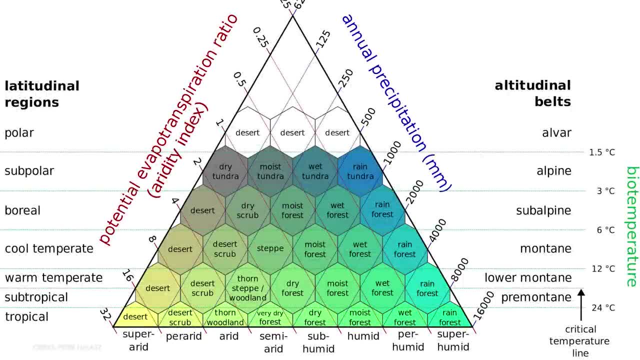 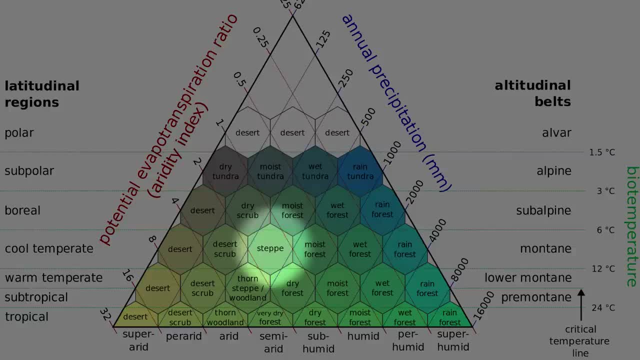 being represented here. If we consult our Holdridge Lifestones chart, we can find the grasslands in the centre as steppe, where conditions are neither particularly cold or hot but where overall rainfall is on the drier side, indicating that grasslands can dominate. 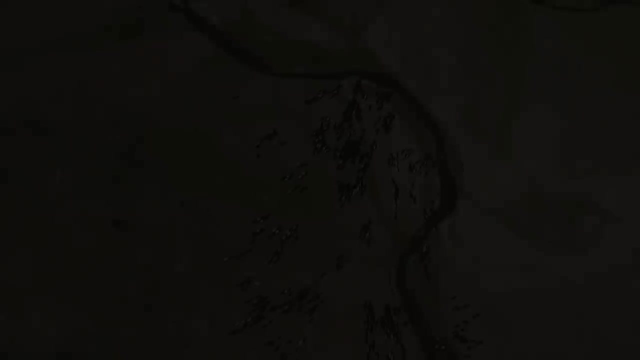 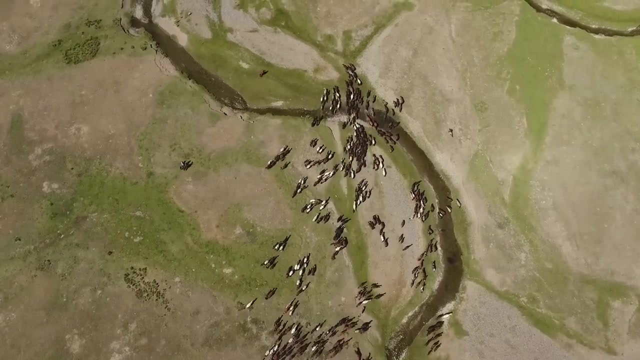 in these more arid areas where trees might struggle. So you've probably heard the terms prairie and steppe, and possibly pampas and veldt too. These terms are more regional in usage than technical. Prairie is almost exclusively used to refer to the grasslands of North America. 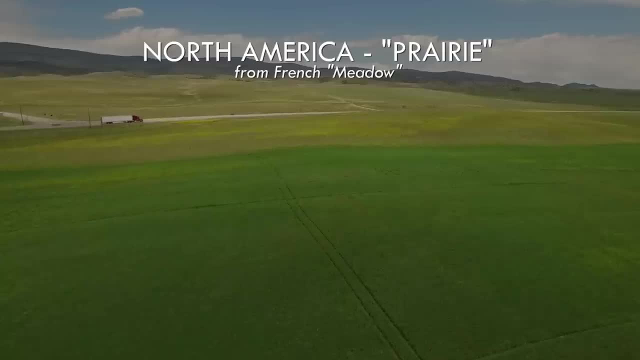 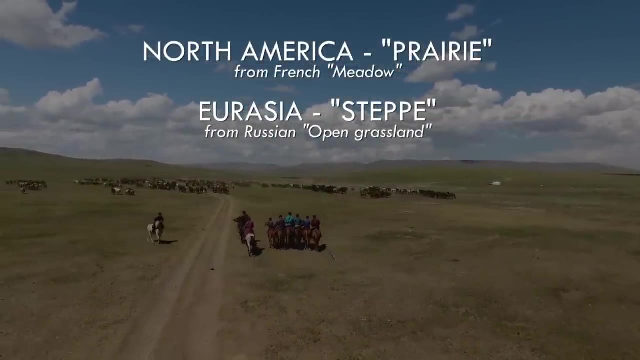 and is a word borrowed from the early French settlers to this region, meaning simply meadow. in that language, Steppe refers mostly to the grasslands of Eurasia and is taken directly from the Russian word for this, biome. Pampas is the most common word. 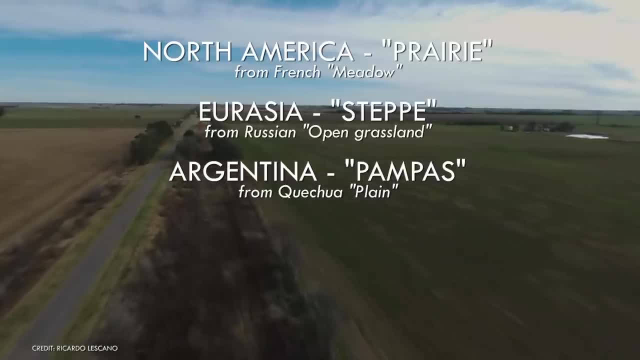 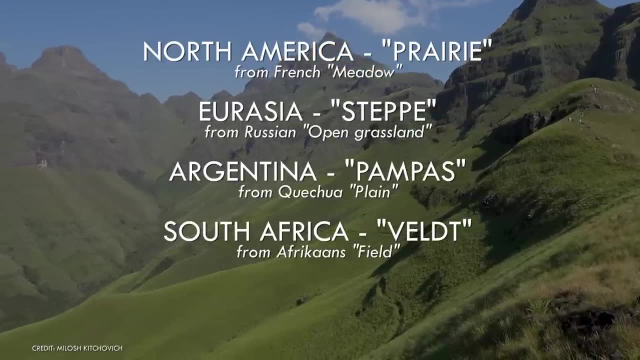 for the extensive grasslands of mid-southern South America and is from the catch of a word for plain Veldt. the Afrikaans word for field is a loose term used to describe the open upland country of East and South Africa. 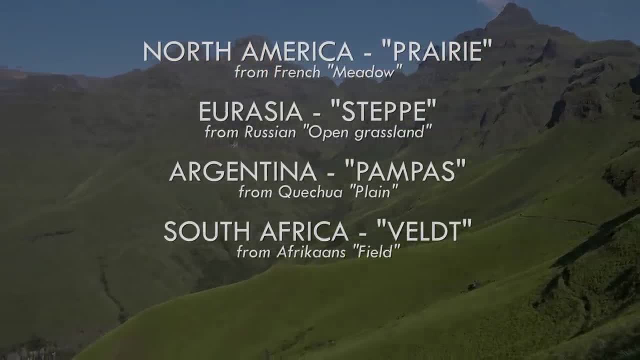 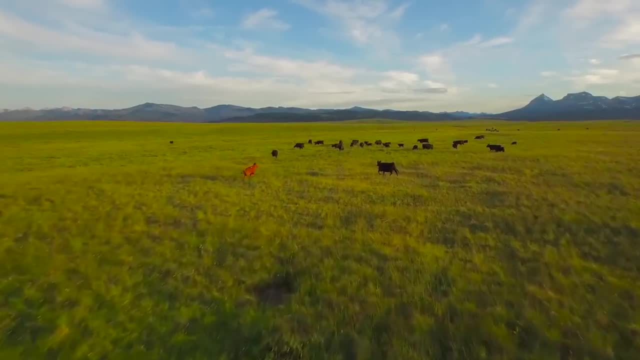 that is sometimes grassland, but might also be scrub. Beyond the vernacular terms, grasslands vary more technically in the height of grass And in the absence of grazing animals. this relationship is determined by the amount of rainfall and soil drainage. Where the soil is wetter, 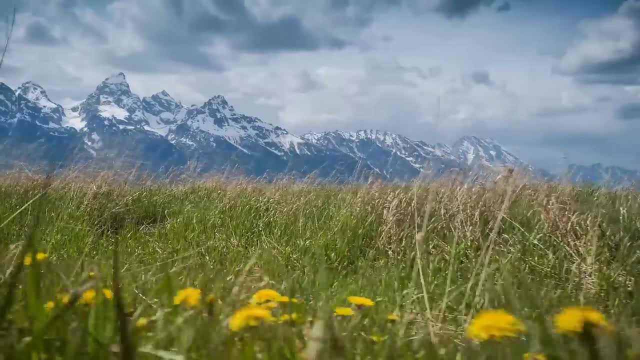 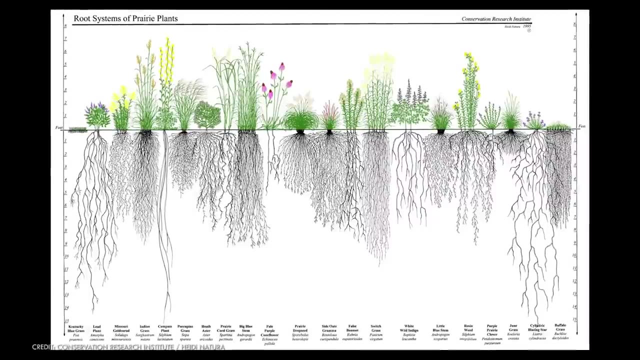 the grasses will grow taller, with some species growing up to 4 metres in height, while more arid conditions lead to shorter grass. Anyone who has tried to dig up the turf or sod of their lawn will know how well grasses bind to the soil. 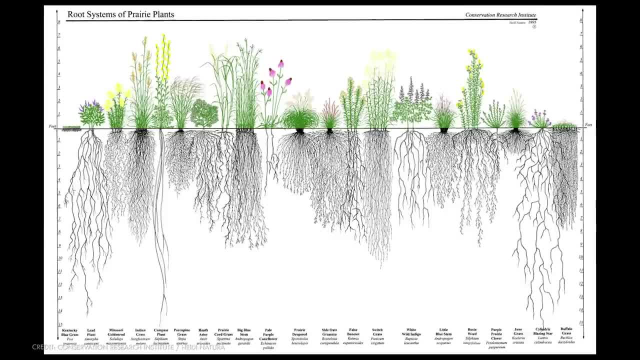 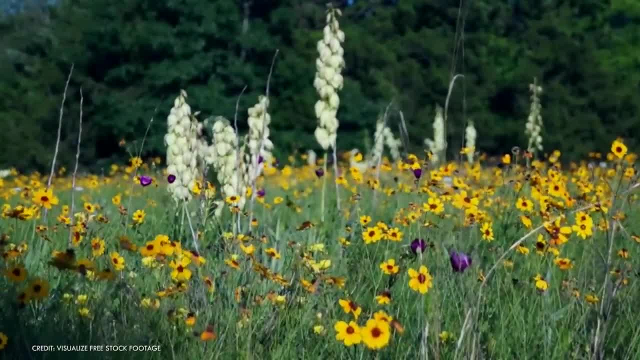 and the tall grass species also follow this pattern, with roots burrowing into the earth as deep as their structures are above ground. As grasses are flowering plants, meadows burst into vivid colour during the season of plant reproduction, which occurs in the spring in the mid-latitudes. 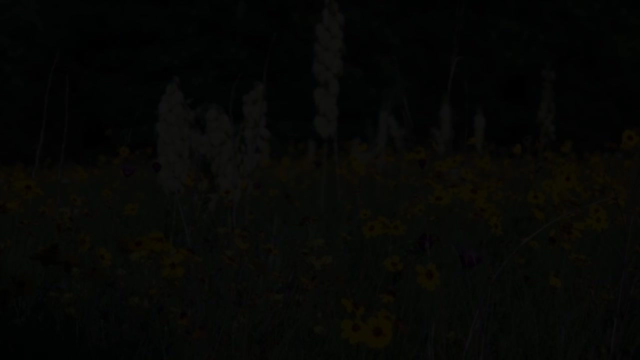 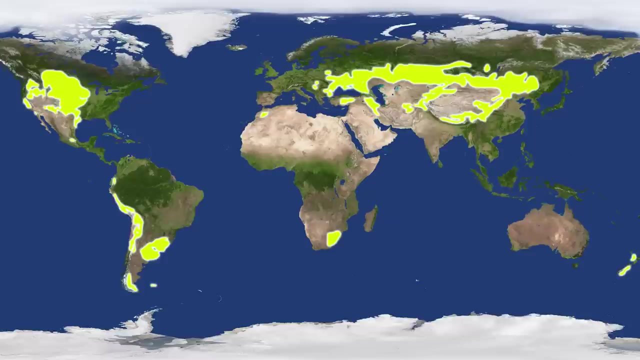 and at the beginning of the wet season in subtropical highland areas. So where in the world do we find the grasslands? The two northern continents of North America and Eurasia form most of the land area of this biome, with the Great Plains of their heartlands being made up of prairie and steppe. 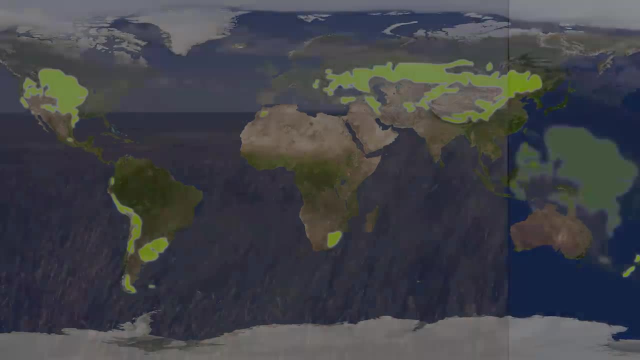 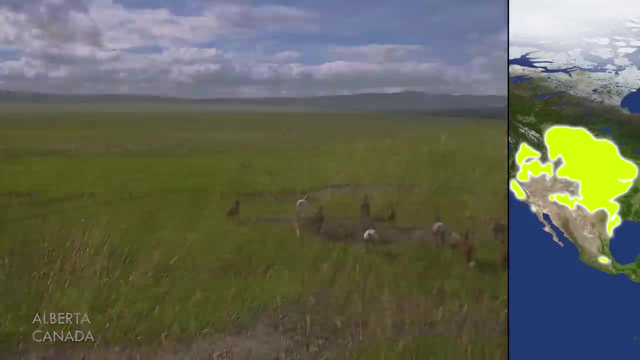 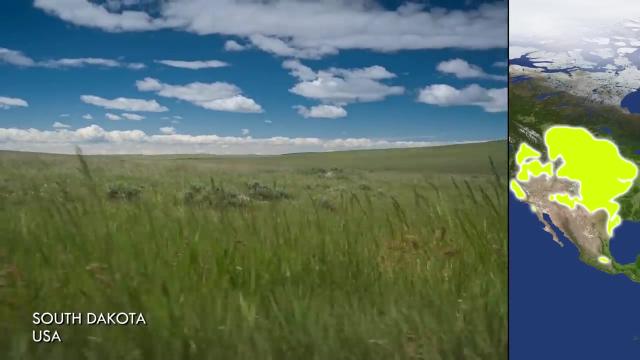 The southern hemisphere, by comparison, has more isolated areas. The North American prairies extend unbroken in vast plains from Alberta, Saskatchewan and Manitoba in Canada, south and east into the central part of the United States, including the states of Montana, the Dakotas, Minnesota, Wyoming. 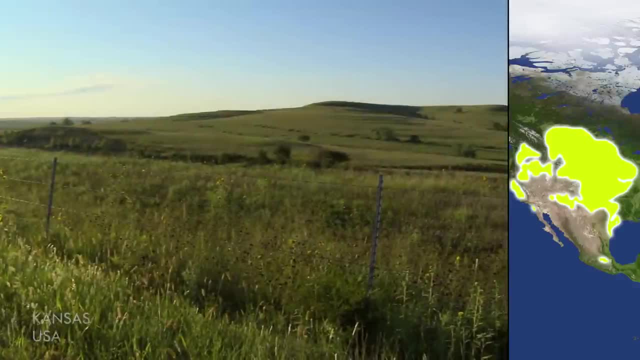 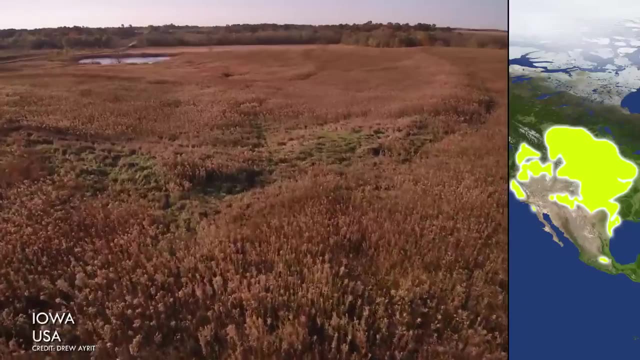 Nebraska, Iowa, Kansas, Missouri, Oklahoma, New Mexico and Texas. In these regions, the eastern parts receive more rain and are naturally tall grass prairies which blend into the temperate forests of the eastern part of that continent As we travel west toward the Rockies. 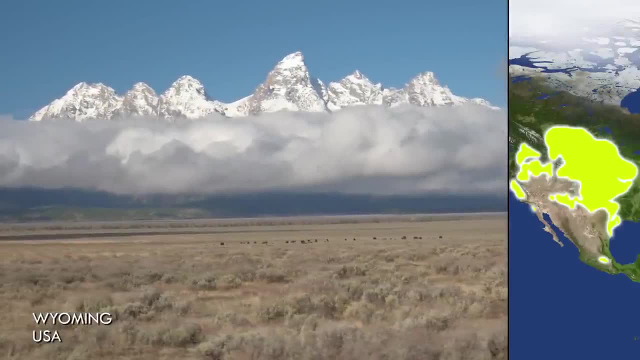 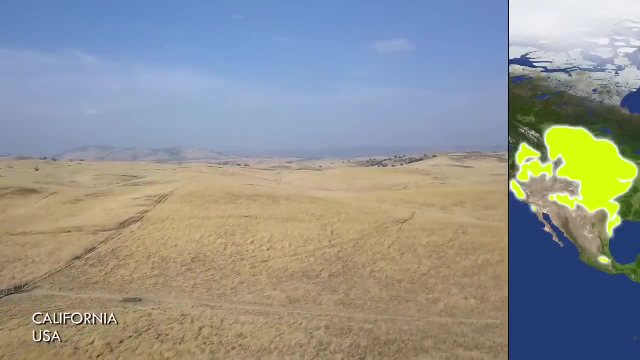 less rainfall leads to shorter grass until semi-arid and scrub conditions occur. Parts of the high desert of Washington, Oregon, Idaho and Nevada have grassland, as does the low-lying Central Valley of California. In practically all these areas, however, 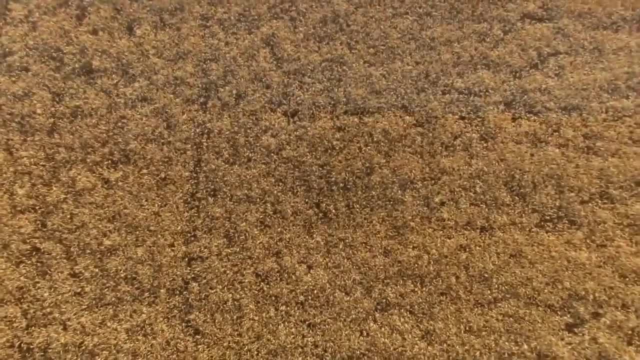 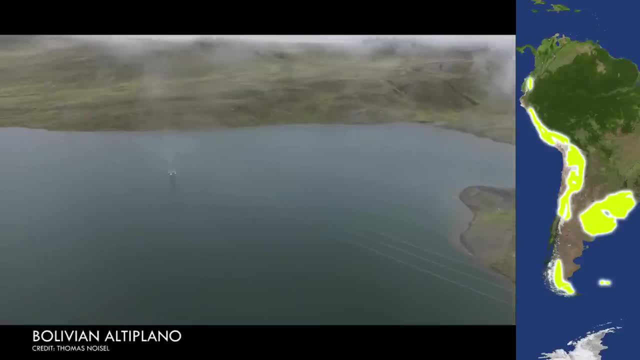 the excellent soils and suitability for wheat and corn farming have led to the decimation of natural prairie, with very few areas remaining. South America has three areas of grassland. The first, known as Puna, can be found in upland subtropical areas. 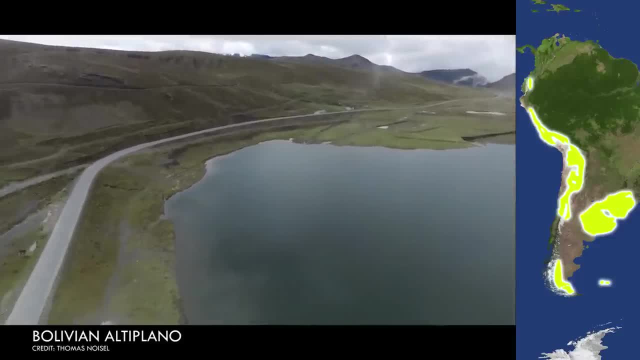 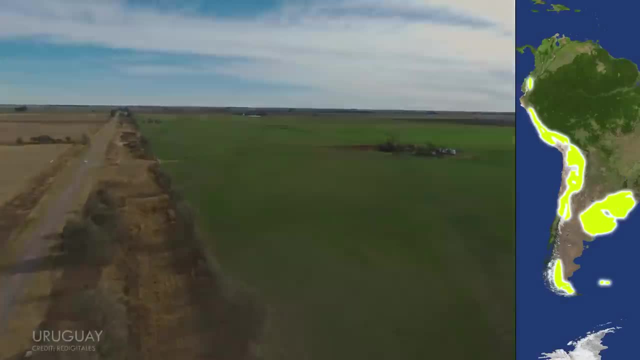 of the Andes, where much of this remains preserved in its natural state. It's a different story for the pampas of northeastern Argentina, Uruguay and southern Brazil, however, where the extensive pampas has been converted almost entirely to farming. 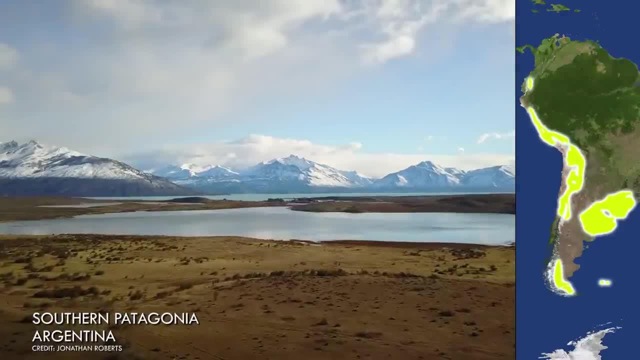 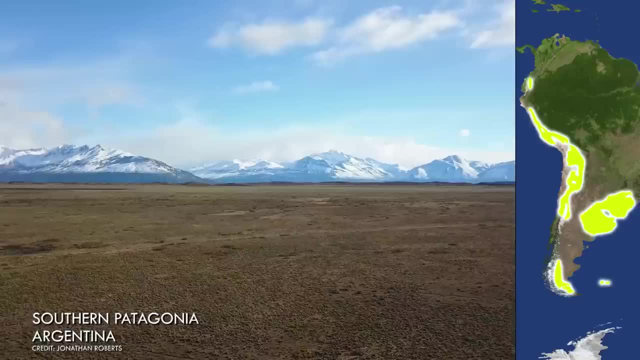 with ranching dominating. Lastly, the eastern tip of this continent, from Tierra del Fuego to southern Patagonia, as well as the Falkland Islands, are dominated by grasslands in the most polar latitudes of any in the world. 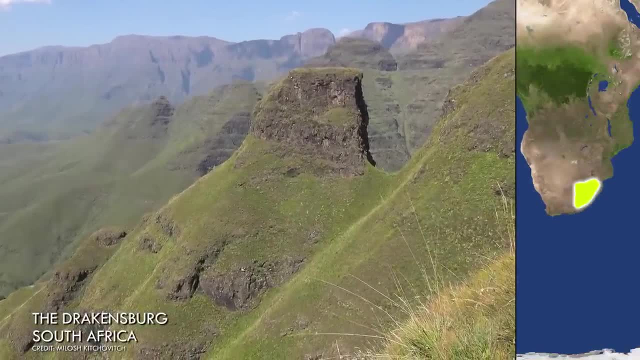 In Africa, that continent, dominated by the tropical winds, is known as the Pampas of the Andes, dominated by the tropical savannah. Only a small portion of it, in eastern South Africa, is considered a part of the true grassland biome. 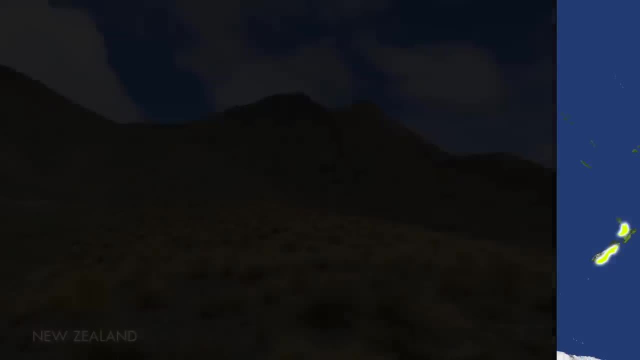 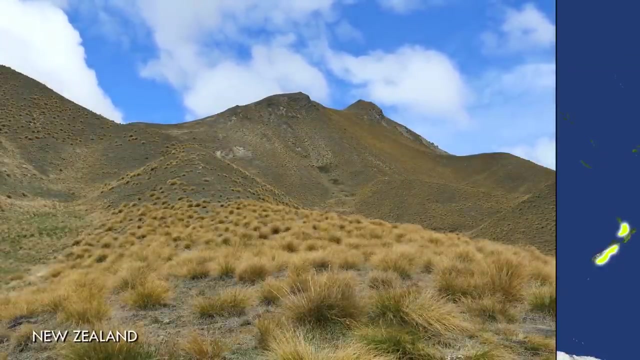 found in uplands, where it is known as the Veldt. We find a surprising area of natural grassland on both islands of New Zealand, a country otherwise dominated by temperate forests owing to its oceanic climate. The causes of these tussock grasslands? 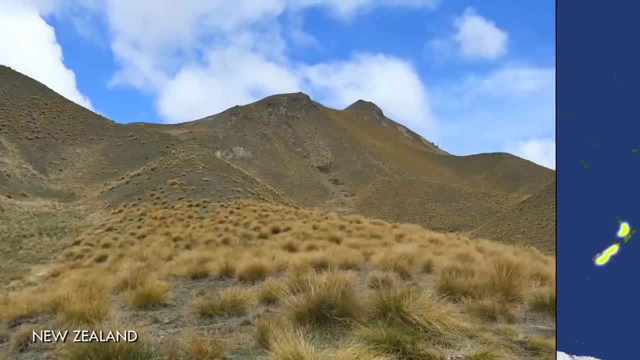 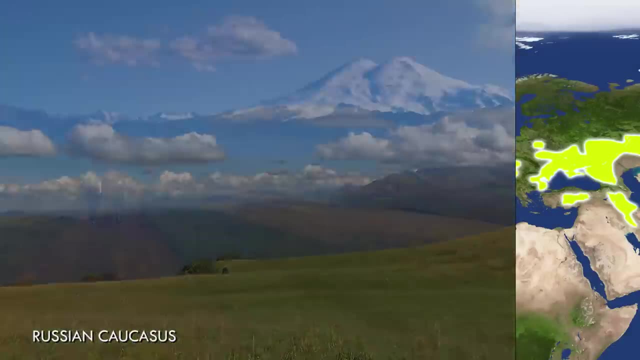 are poor soils in the centre of North Island and a rain shadow in the South Island east of the Southern Alps that reduces rainfall significantly. In the Middle East we have relatively isolated pockets of grassland in upland areas of Turkey and the Southern Caucasus. 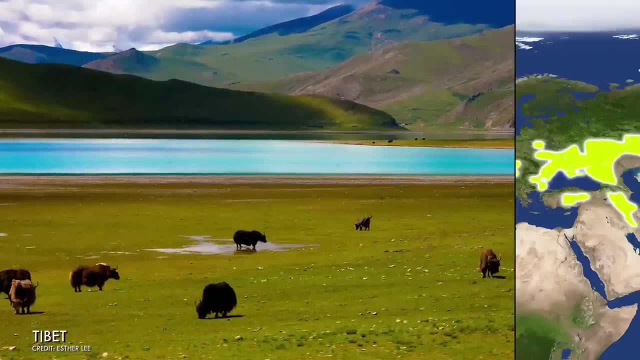 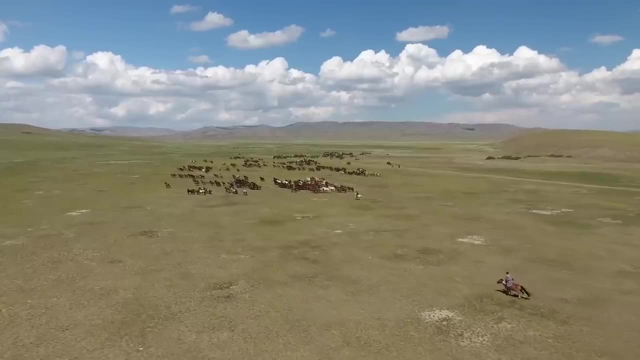 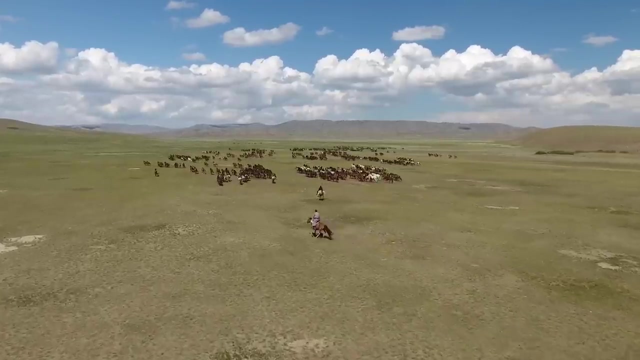 while mainly subtropical areas surrounding the Tibetan Plateau have this biome in a similar way to those of the Andes, However, these areas pale in comparison to the largest area of grassland on Earth, the vast steppe plains of Eurasia, Running in an unbroken line at around 45 degrees north in latitude. 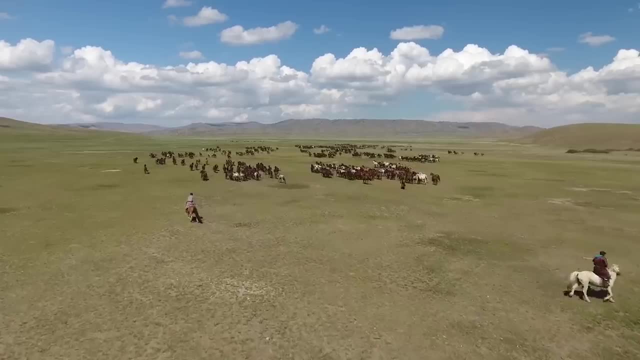 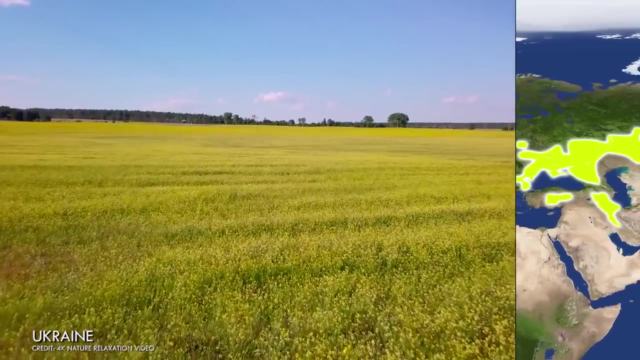 the steppe separates the temperate and boreal forests of the north from the deserts of the south. The steppe is the largest of the continent. in Eastern Europe they encompass the whole of Ukraine and the southern half of European Russia, where most of the natural steppe has been transformed into the wheat belt. 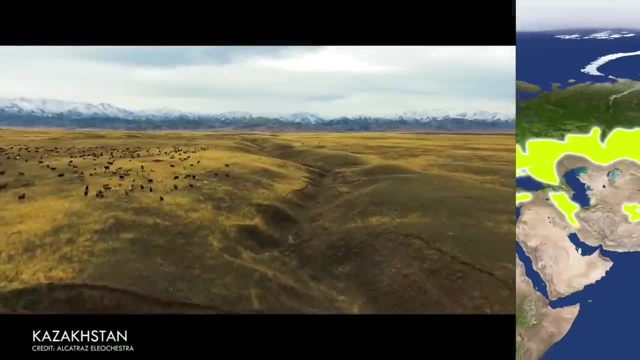 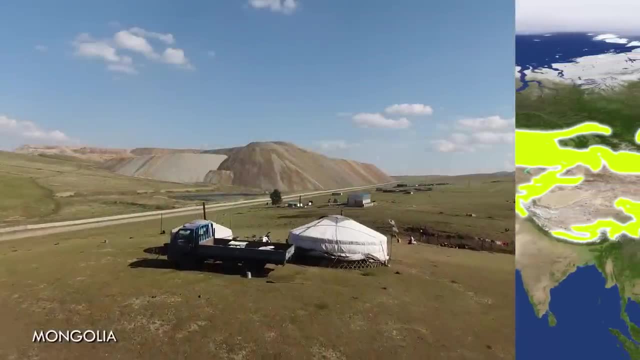 that feeds these countries in a similar way to that of the North American prairies. Further east, the steppe runs along the boundary of Russia and Kazakhstan, and then east again, ending with the border of Mongolia, where the northern half of that country is dominated by steppe, still mostly in its natural state. 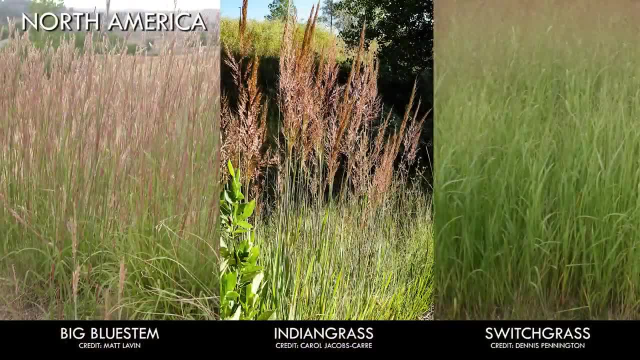 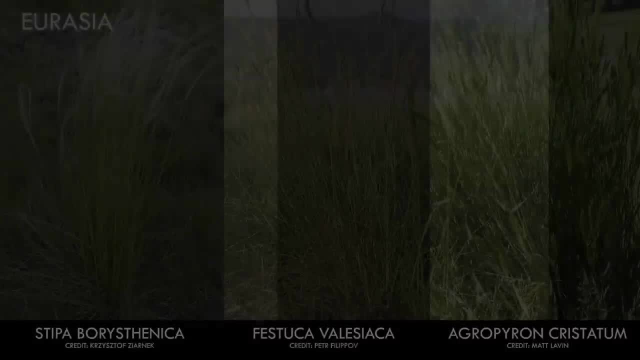 Species. diversity in natural grasslands is high. In addition, we find in the North American prairie, among others, big bluestem, Indian grass and switchgrass species. In the Eurasian steppe, common species families include stipa vestuca and agropyrone. 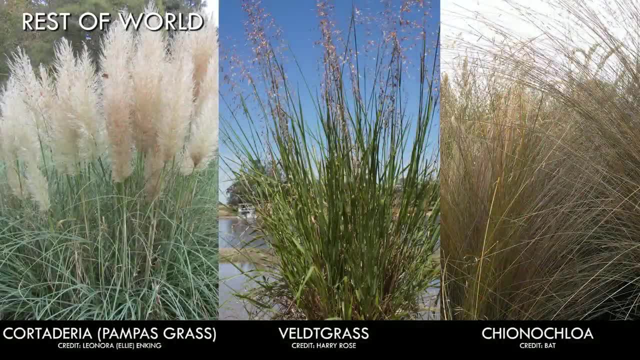 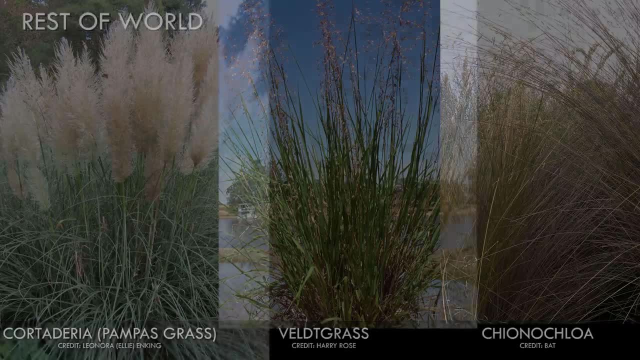 The eponymous pampas grass is found in that South American grassland, while the equally eponymous veldt grass is from South Africa And in the New Zealand tussock grasslands, Chianocloa is common, Like the savannahs of Africa, the presence of large areas of edible grass in the prairies. 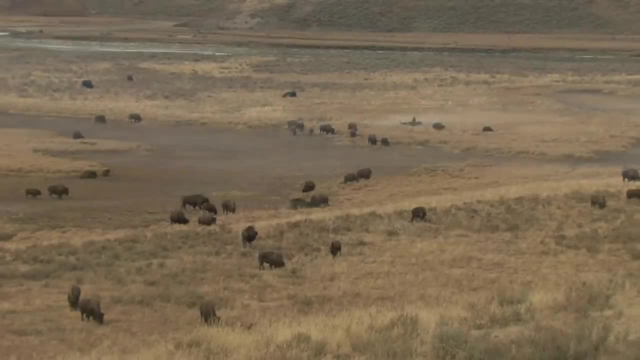 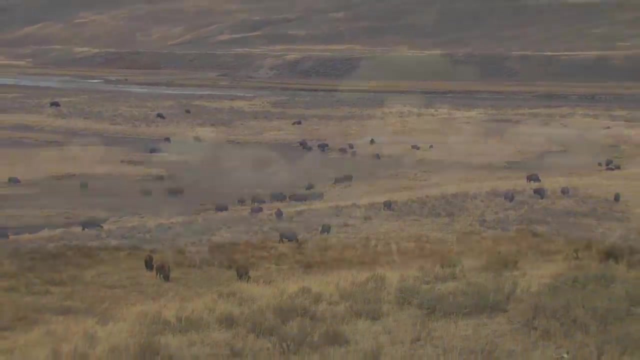 have resulted in the support of vast herds of grazing animals. In North America, there were once tens of millions of bison roaming the prairie before the mass slaughter of the 1800s, And let's not forget that the grasslands of North America and Eurasia led to the evolution.